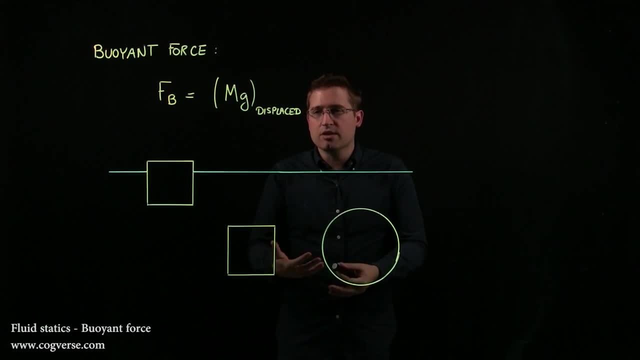 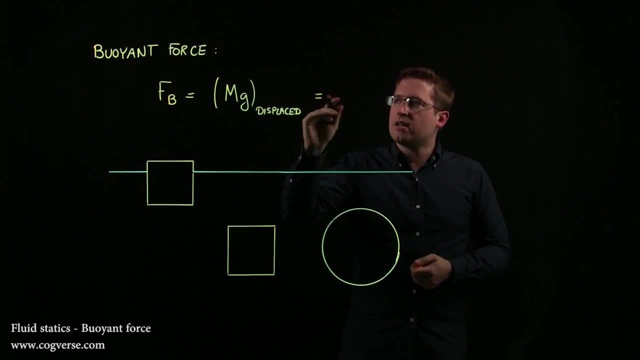 and we can evaluate its weight. So that's what it means when we say that the buoyant force is equal to the weight of the buoyant force. It's equal to the weight of the displaced fluid, But one better way to write it, because 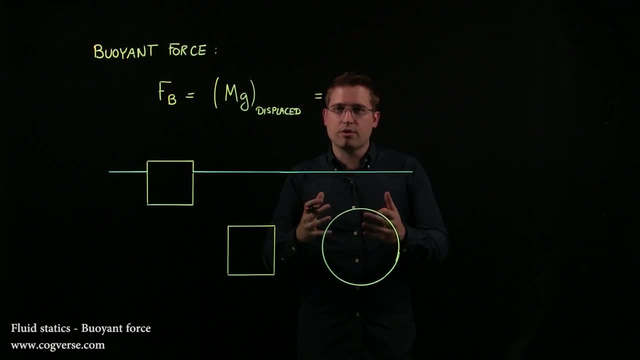 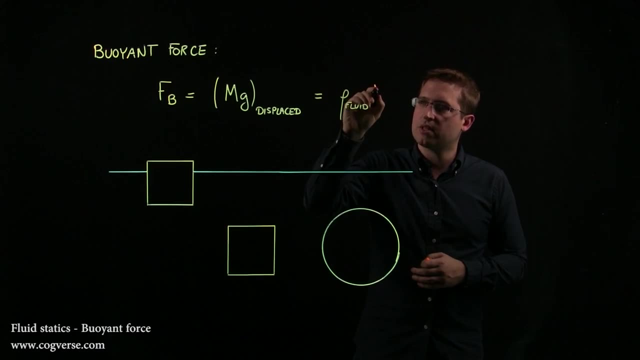 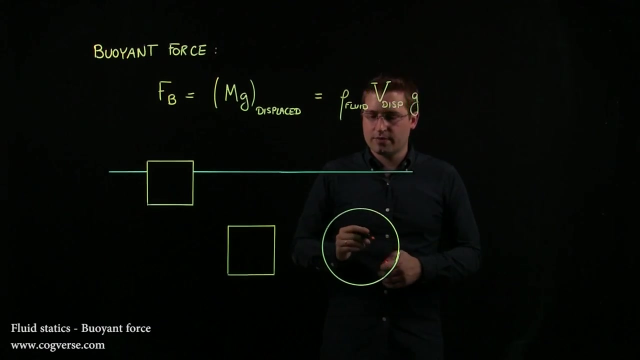 mass is not the best quantity to use. we'd rather use mass density. with a fluid we can write this: rho of fluid times: the volume of the displaced fluid times, g. That's fine. This rho fluid v, displaced, is the same thing as m. 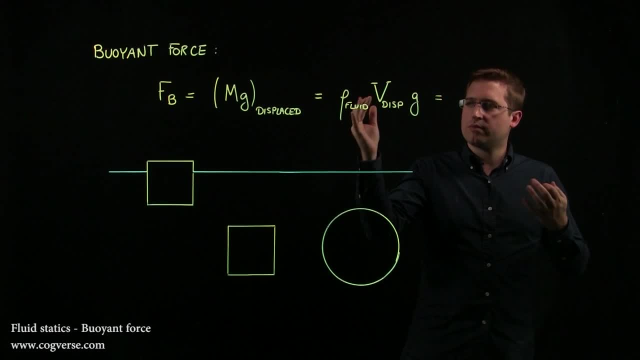 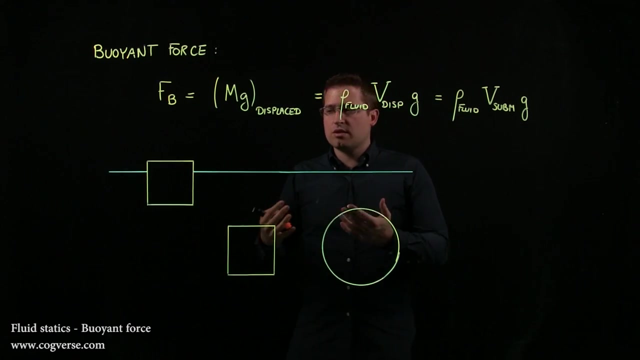 I prefer to use another one, but you can pick the one that's best for you. I use rho fluid v submerged times g. That's just because it's easier to me to visualize the submerged volume of the object rather than the displaced volume of water in this case. say So what? 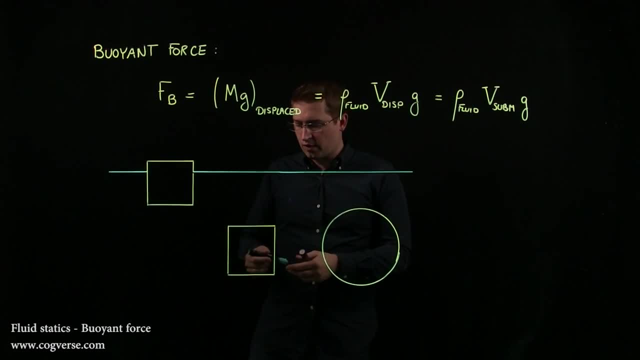 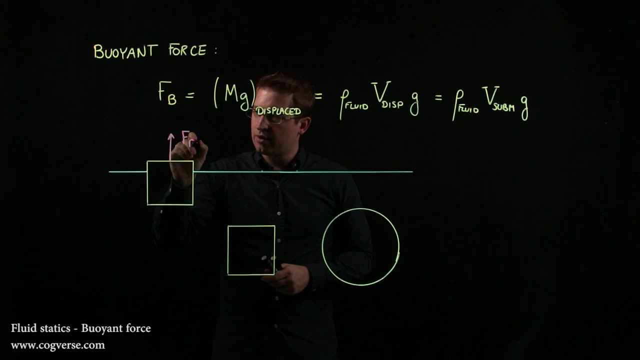 do we mean by rho- fluid v- displaced. Rho fluid v- submerged g? Well, take this block. The buoyant force acting on it is upward, That's how it floats. And the submerged volume, or the volume of displaced water think of. 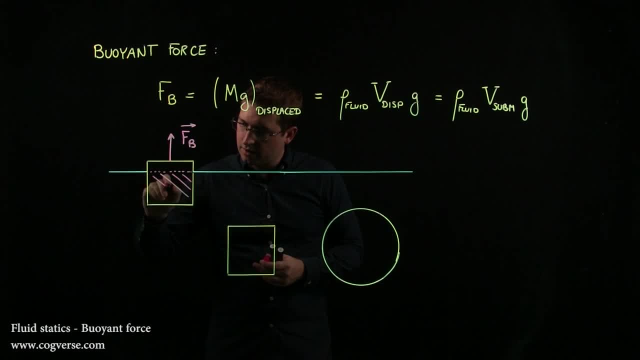 it as you want is all this. And if the bottom has an area a and this is a depth h, then v displaced or v submerged—same thing—is equal to a times h And therefore the buoyant force and magnitude is going to be equal to rho of water: a, h, g. So that's the buoyant. 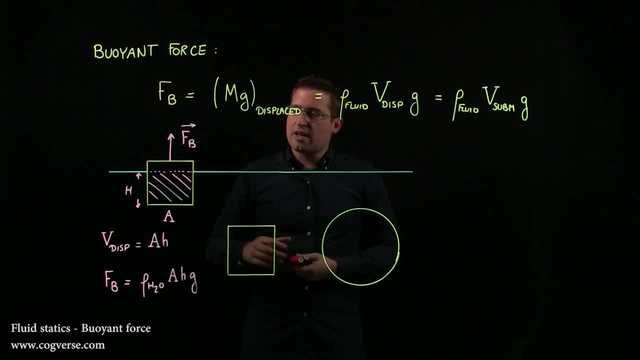 force for this cube, Humモn. Now, what's interesting, though, is that Can we write this, m увеличed by h times: g zabulei? this cube floats, with some of it outside of the water, And what it means is that we could make the buoyant force even bigger. 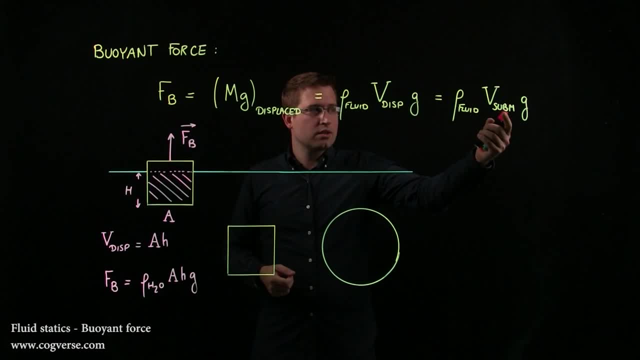 if we somehow pulled down on the cube and submerged more volume, like this one, for example? This cube is entirely submerged And so the entire volume of the cube- let's call it V cube- is the submerged volume. That means that the buoyant force acting on this cube